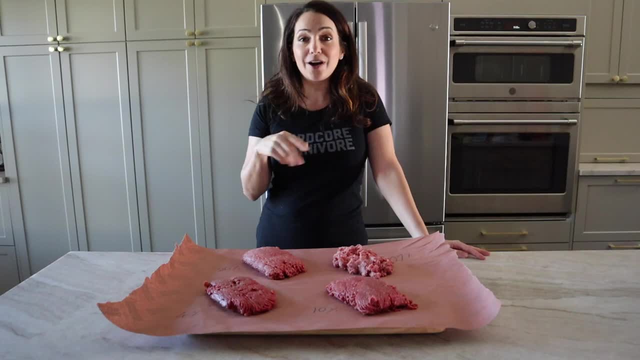 kinds here. These are the ones available in my local grocery store, and actually this is pretty important. if you grind your own sausage, Let's say if you're a hunter like me, you need to understand about what the fat is going to do. So from from down here, and you can see the color difference too. 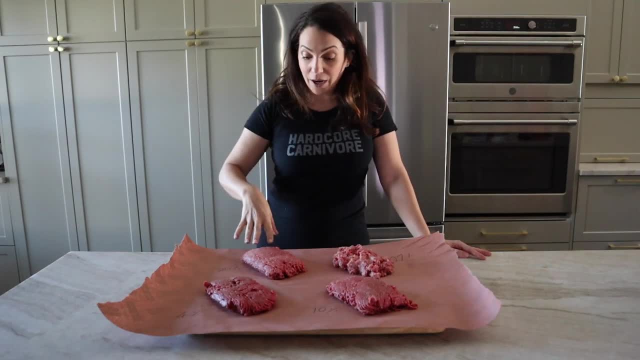 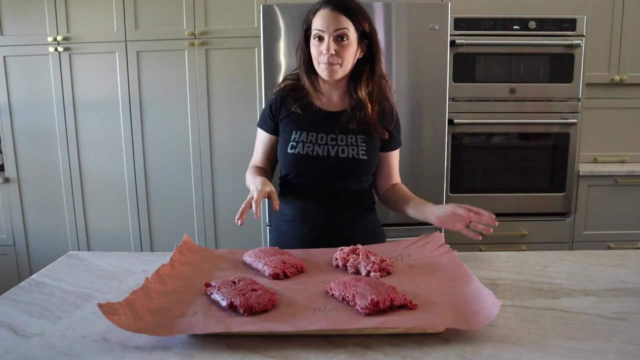 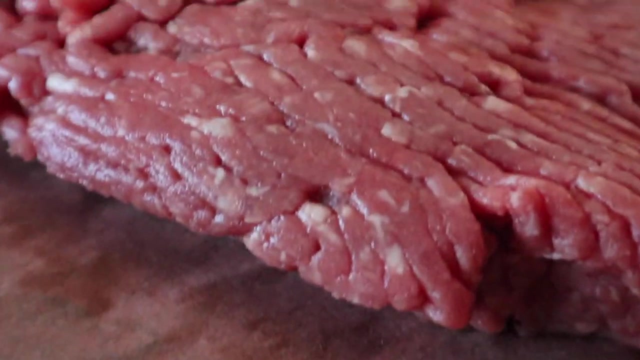 we have a 4%, a 10%, a 20% and a 27%. So 4% fat, 10% fat, 20% fat, 27% fat to lean meat And you can see a huge difference in the gradation of color. from the 4% We get a little bit lighter. 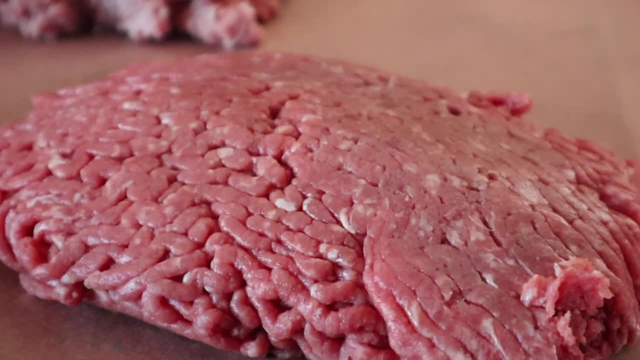 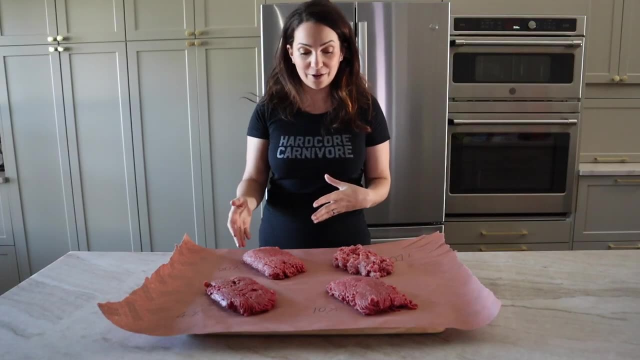 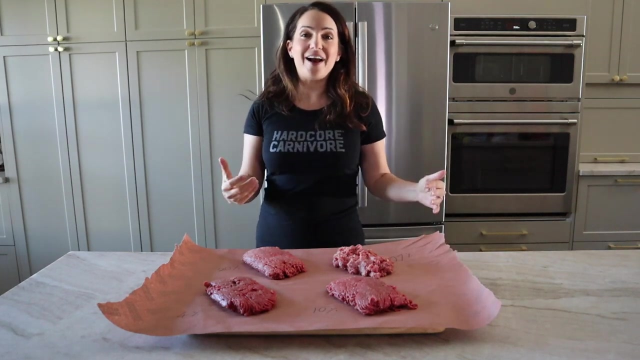 with the 10%, even more lighter with the 20%, and then into kind of a mash with the 27% which, in fairness, came out of one of those tubes rather than on a foam tray. But muscle is going to be that red color and fat is going to be white. So you can expect, as the percentage of fat in your grind goes. 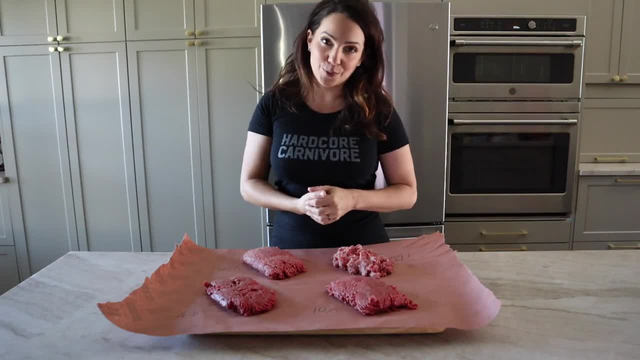 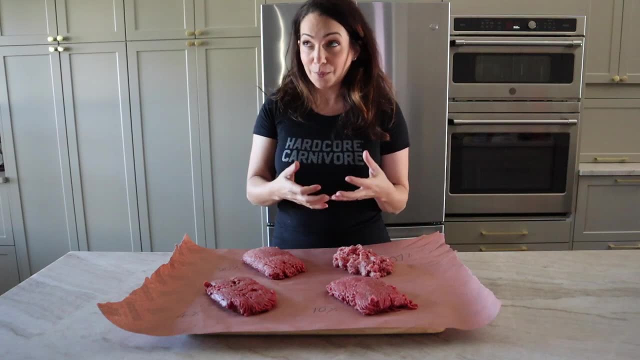 up. the color is going to change too. Why is this important? Okay, so the 4%. this would be for someone who's looking for very lean beef. It's probably for dietary purposes, because this is also going to be much more expensive than, let's say, a 20% or a 27%. 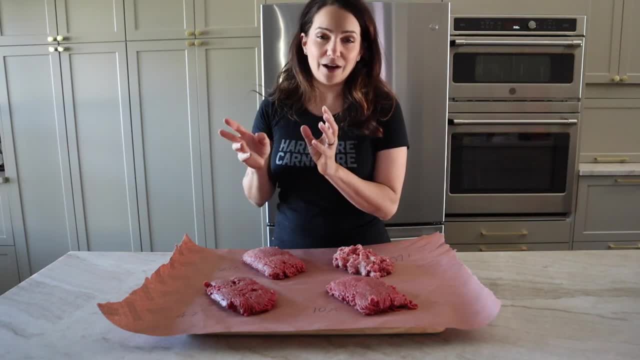 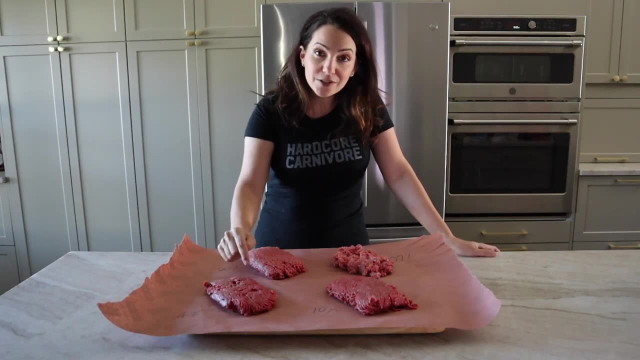 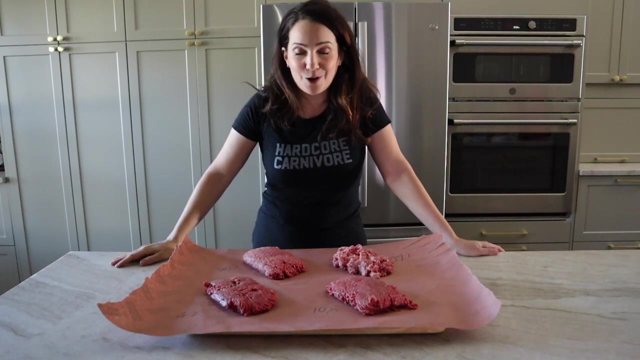 So this is going to be for someone who's looking specifically for lean options and to keep that fat percentage down. If you try and make something like meatballs or a burger using a 4%, this right here is why you will have a dry result. Fat is so important. 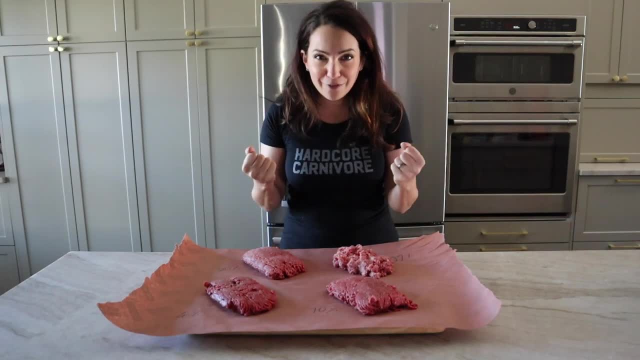 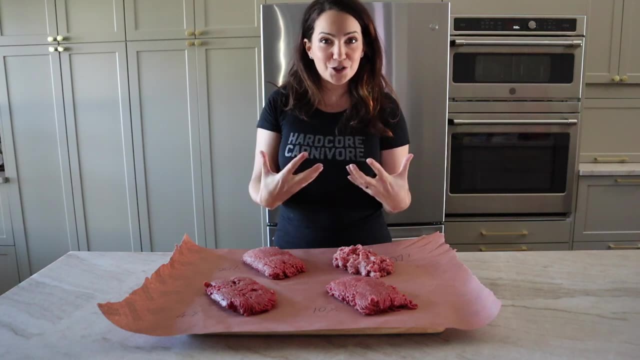 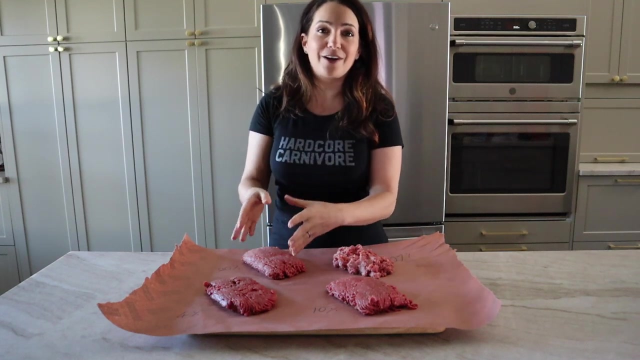 It's crucial, not only as a vehicle for flavor, but that's where your moisture is going to come from, All of that beautiful rendering fat that cooks out during the cooking process. So when you've only got 4% of fat, you're going to have so much different a mouthfeel and an eating. 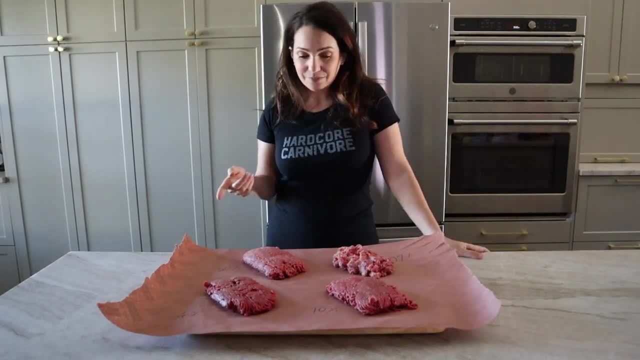 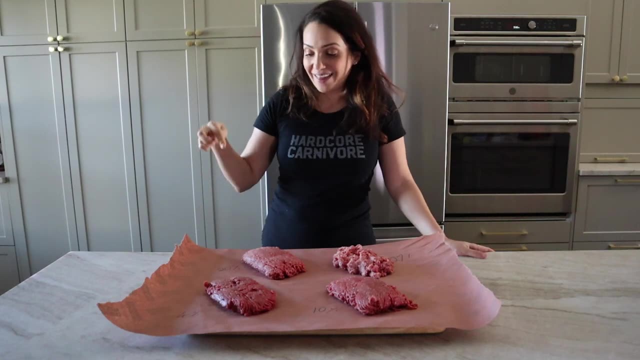 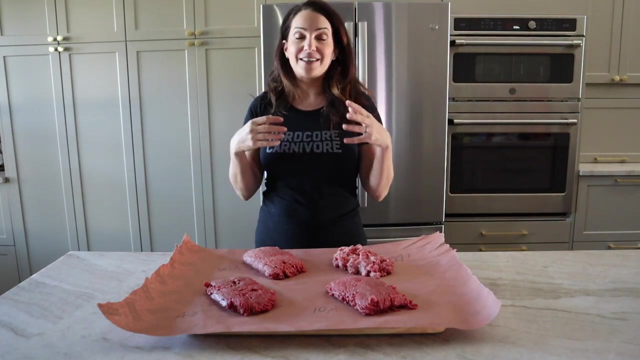 experience than when you're dealing even with something like a 20%. So for burgers especially, particularly if you're looking for that juicy result, I would go with at least a 20% all the way up to maybe, you know- a 27%, maybe a 30%, because that's what's going to. 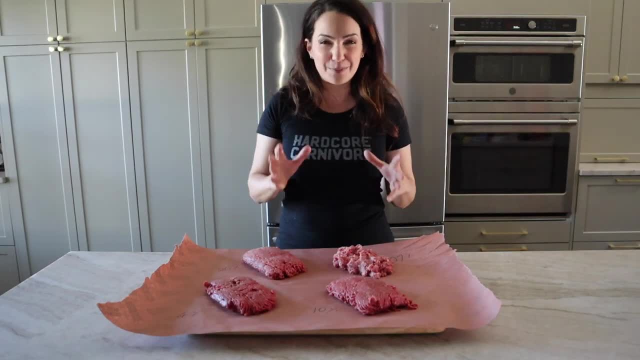 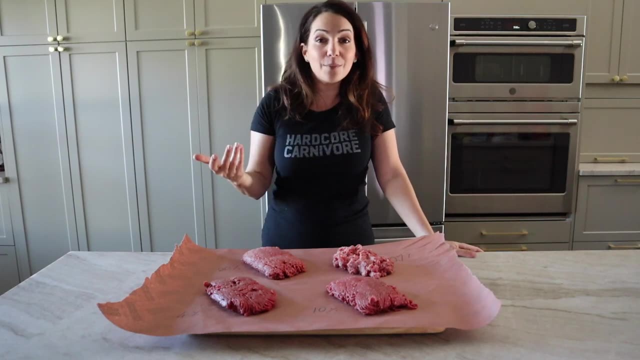 keep it juicy. And even if you're like me and you really like those smash burgers, the ones that are flattened all the way on the griddle, that fat percentage is still going to help because, if you think about it, instead of like a 20% fat percentage, you're going to want to keep it juicy. 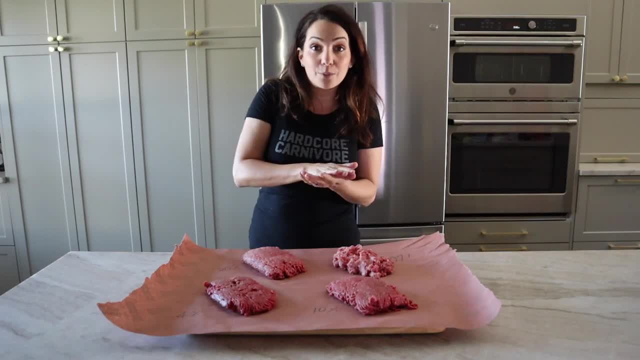 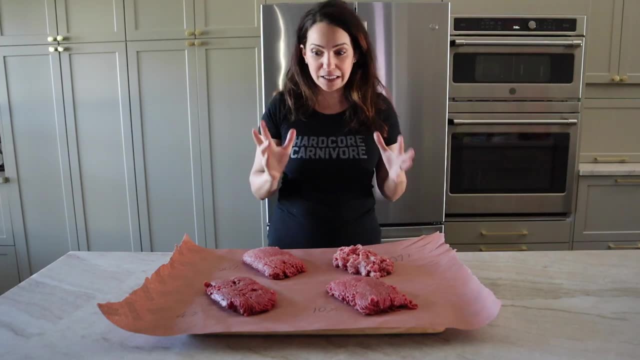 Let's say adding olive oil to the griddle and then putting your beef on to brown, you've got that fat already in there that's going to help get that amazing crust and that amazing sear. So that's the main difference between what these percentages do. but I wanted to talk a little. 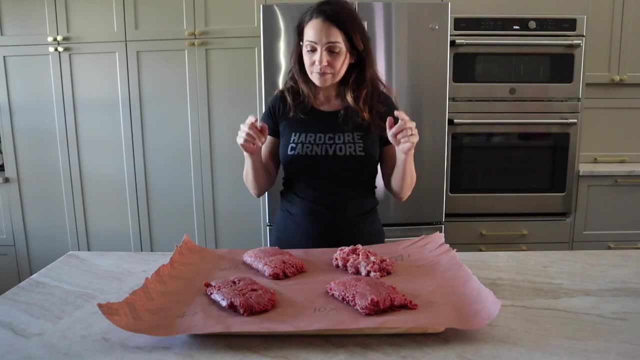 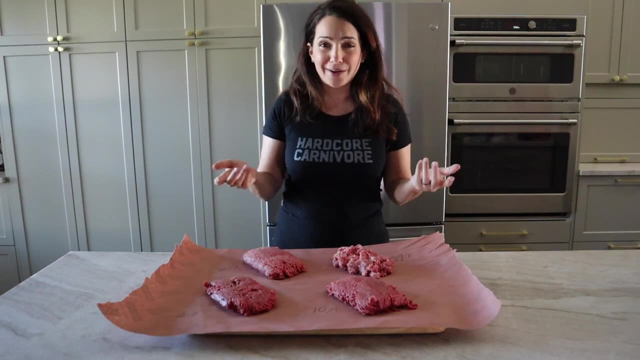 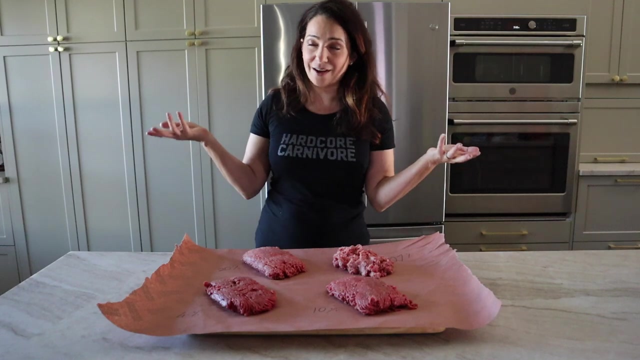 bit about the quality of ground beef. Everything you see here is literally just beef, ground beef, nothing more. nothing added in. there's no breadcrumbs, there's no filler, there's nothing like that, and yet it can get a little bit of a bad reputation. we've all heard the lips and 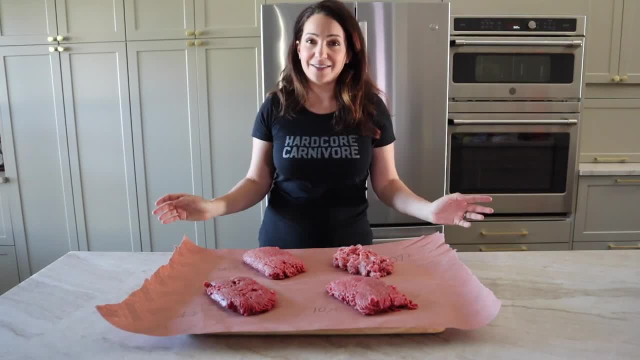 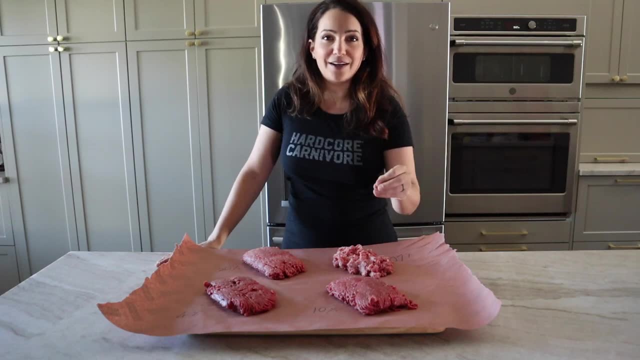 assholes thing, and I can assure you that that is definitely not the case. I've been in enough processing plants to tell you that when you look at cattle as a commodity- and that's what it truly is- it works in both ways okay, because not only are the processing plants trying to treat it as 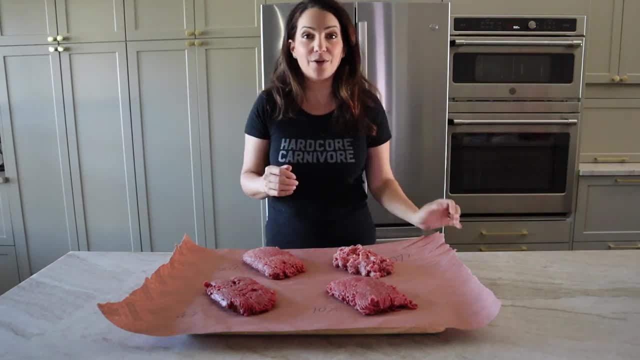 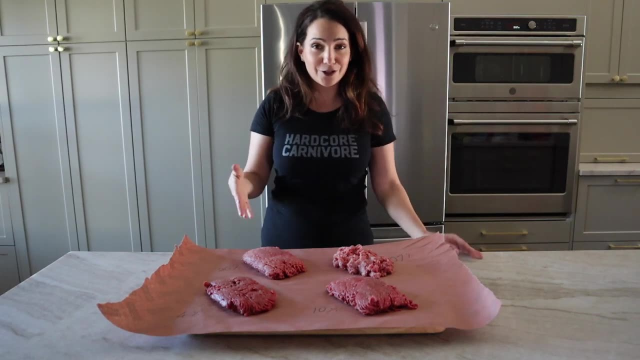 a commodity and get the most value out of that animal, but from a sustainability. they are using every part possible, even the parts you don't see here. so even the bones get turned into render, which can get turned into feed, and a million items for items that you probably didn't. 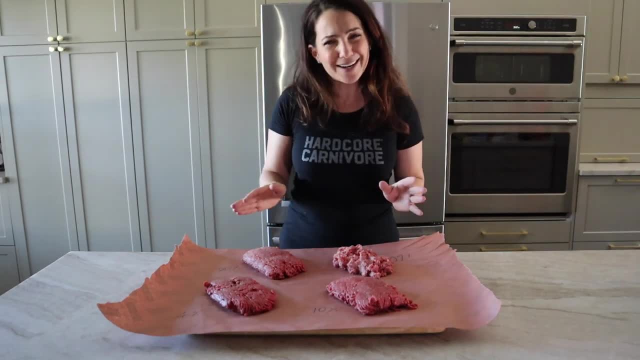 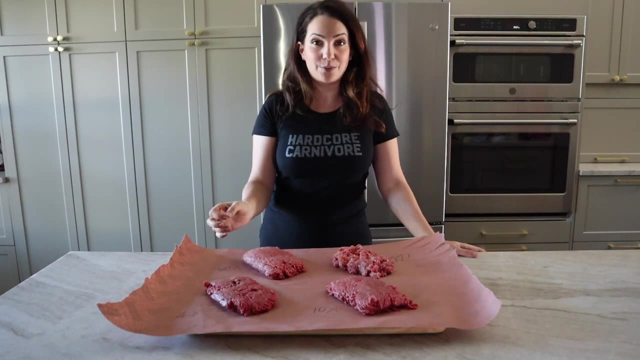 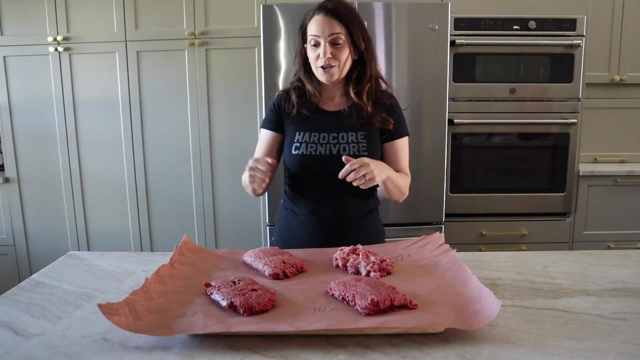 even realize are made from beef. I'm digressing. I get excited about this stuff, okay, but uh, they do want to try and salvage as much meat as possible. so if I handed you some bones to break down or some cuts to break down, the chances are that you wouldn't be able to scrape. 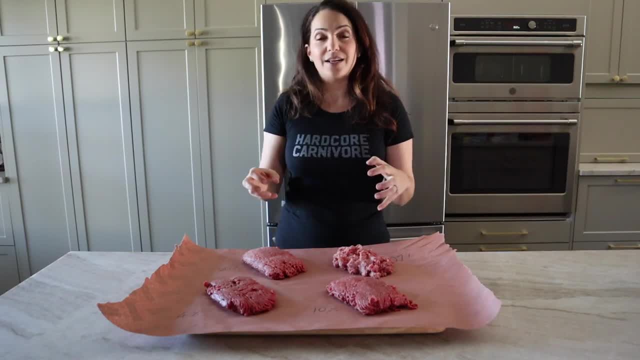 all of that meat off, and the way that we get to grind is those little muscles that you're not going to turn into steaks, extra meat that's left on the bones that we can scrape off and put into here. so it's perfectly edible, it's perfectly normal beef. I hate that it sometimes gets a. 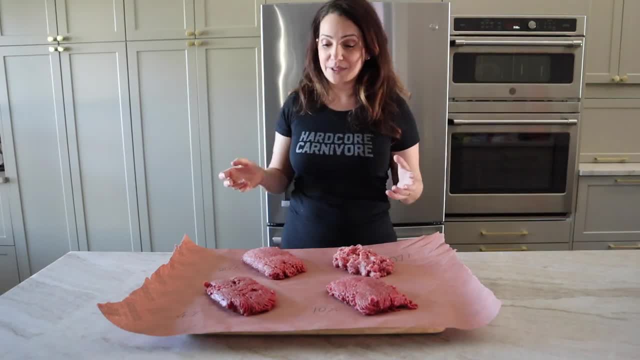 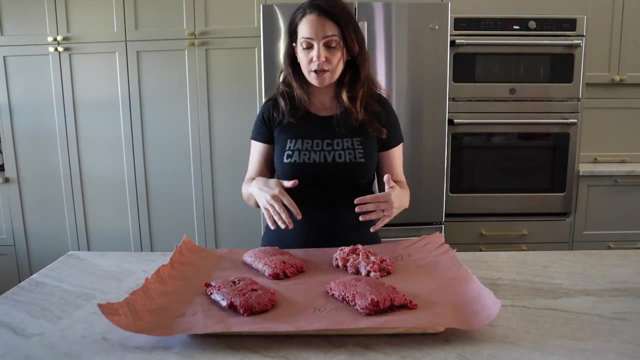 bad reputation, but that's how it is and that's how it's made. so one last thing I want to talk about. so within ground beef especially, and you can see that color gradation. but then you see the this a lot with sausage- PS sausage. you're going to want to stick in this back row with. 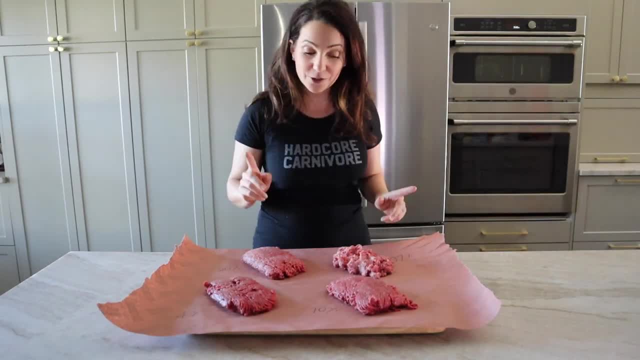 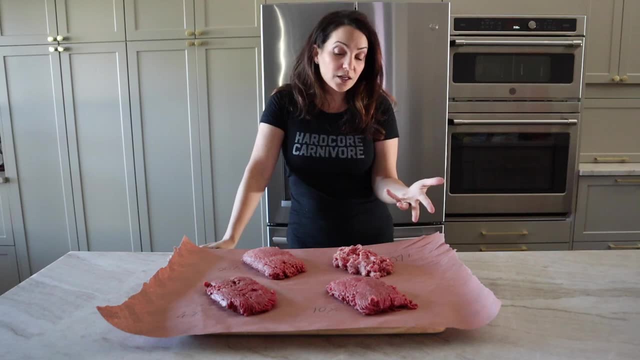 that super fatty grind too to get that nice juicy sausage. but you know, when you're talking about sausage and the quality of it, or ground meat and the quality of it, sometimes you'll be eating, you know, that burger and there'll be that little bit of cartilage, a little bit. 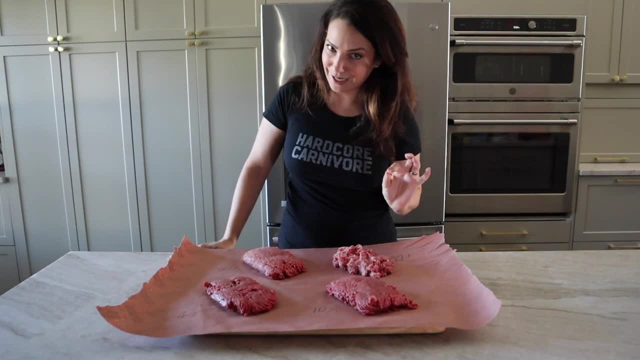 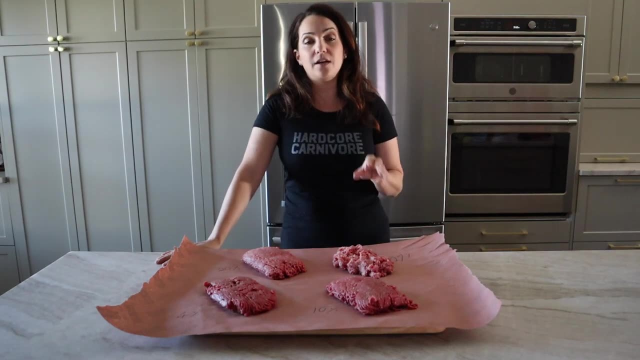 of something, something that you don't want to eat, and you find yourself taken out of your mouth awkwardly, and that's not a difference in how edible it is, that's purely a difference in the quality of what they've chosen to put in the grind. so you hear people talking about 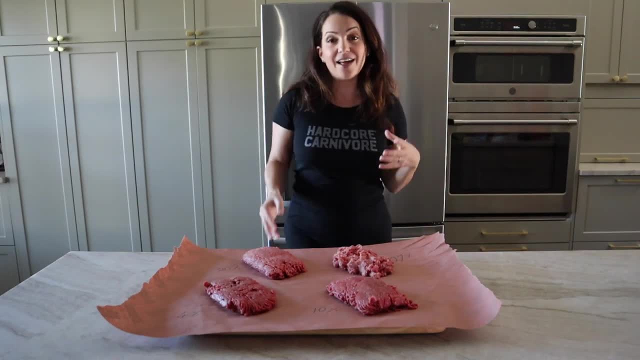 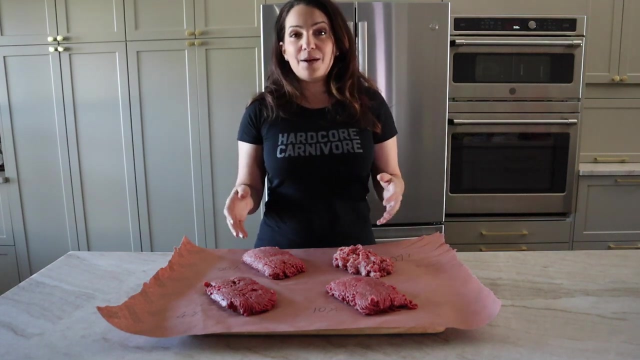 best burgers come from a brisket and chuck mix and that's us taking two whole mussels and grinding them to make a specific, a specific ground mix. right, and when you're grinding whole mussels you're not going to have a whole lot of kind of other junk in there. but sometimes 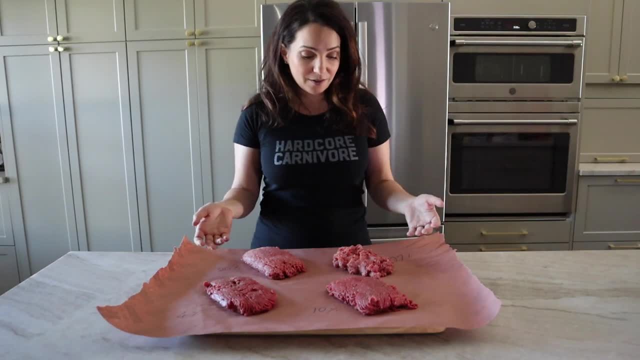 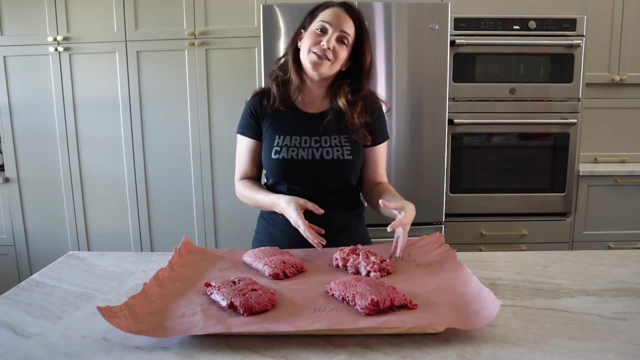 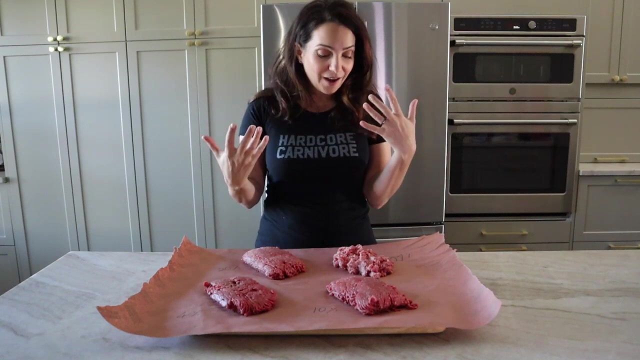 when you're dealing with economical grind too. so, for example, you're 27%. it's not just the fat content in here, but I can see visually that this is a very economical choice as well, which means slightly lower quality cuts and bits and pieces are going to go in there, and when I say bits and 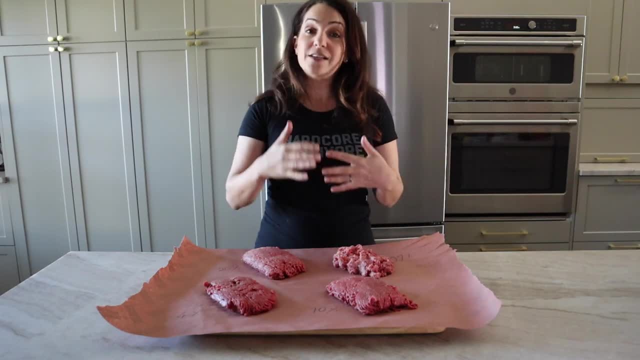 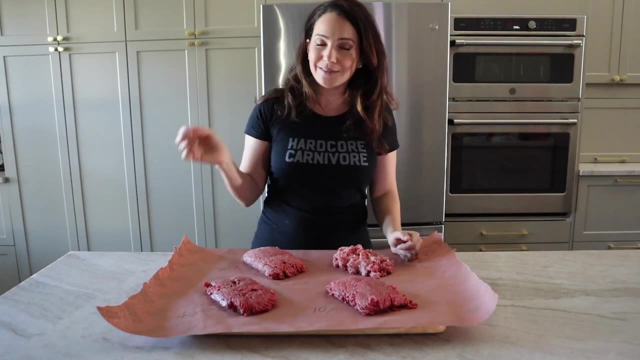 pieces. I want to be clear: that just means there's going to be more silver skin, which is that kind of tough outer layer we see on mussels sometimes. that's the part you're usually- you're usually pulling out of your teeth, and sometimes a little bit of cartilage, again, perfectly edible. 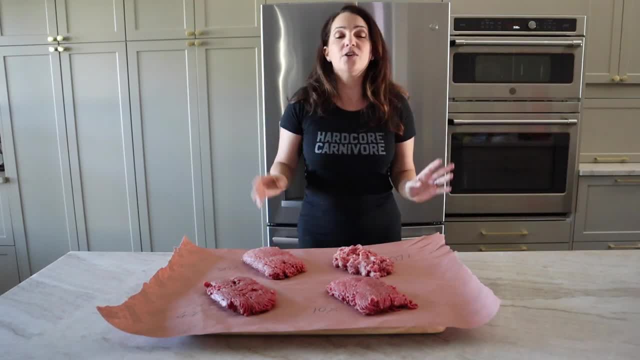 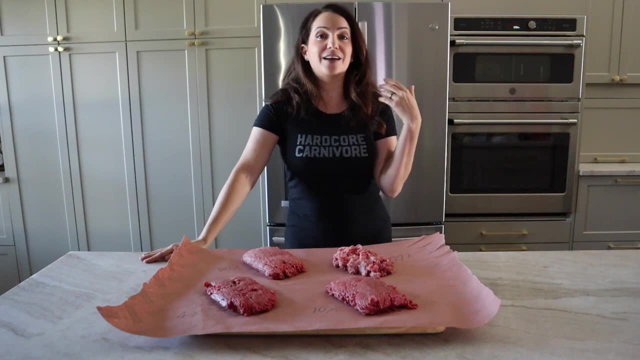 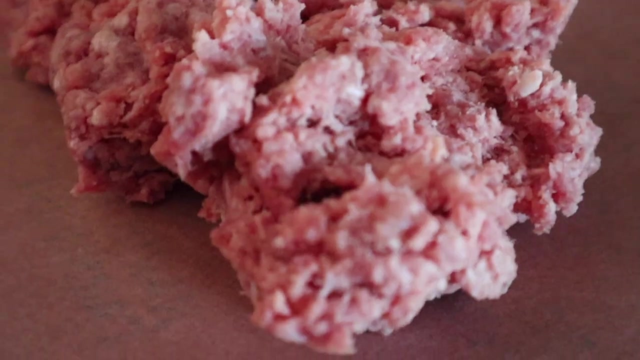 natural part of the animal, but it does make its way into here. so, particularly if you are a hunter, the quality of your breakfast sausage, your ground venison, all of that kind of stuff, is going to depend on how picky you are when you trim your meat. are you doing a good job? 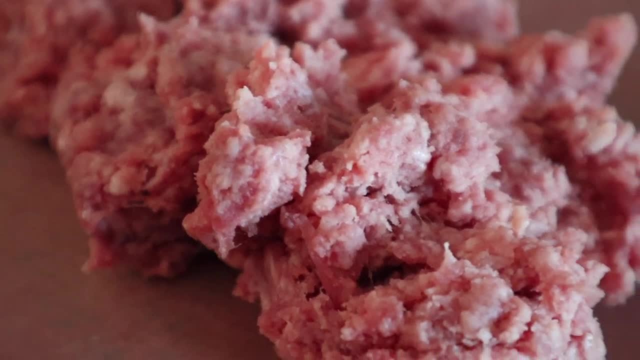 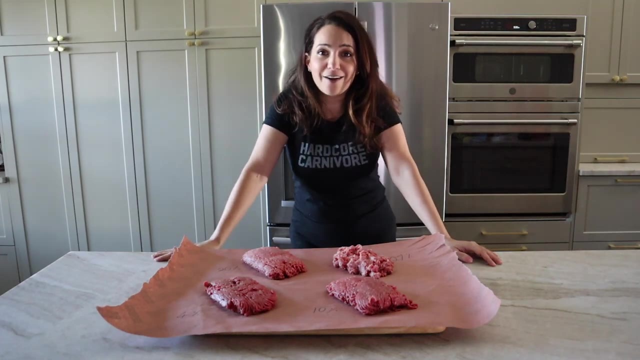 of taking out that silver skin, are you putting premium stuff in there? it'll make a huge difference. so now you know what the four, the 10, the 20 and the 27 are and how you use them all, and I think I'm going to go make me a burger.